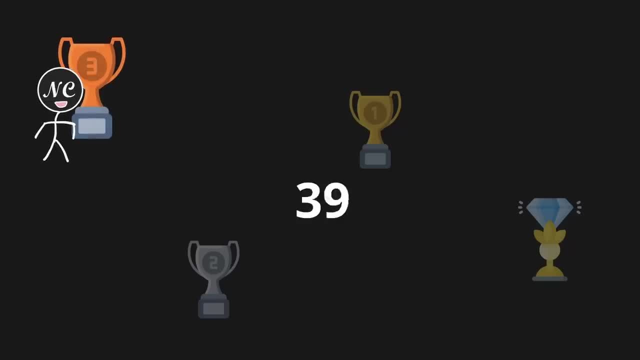 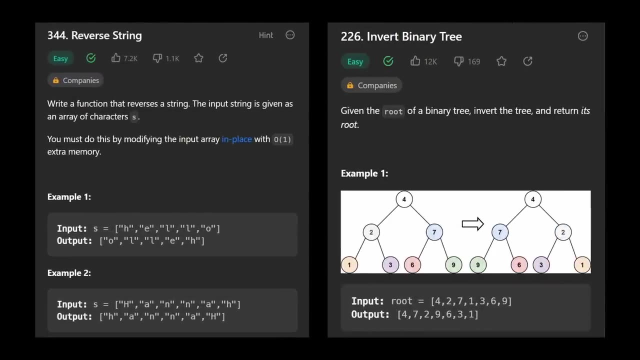 So let's get started. And 50 problems later. that's where I was. I could solve a lot of the trivial problems like reversing a string or inverting a binary tree, but I hadn't even touched a graph problem and I didn't even know what dynamic programming was. But believe it or 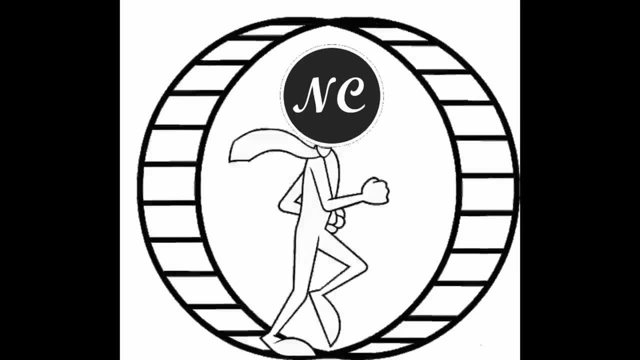 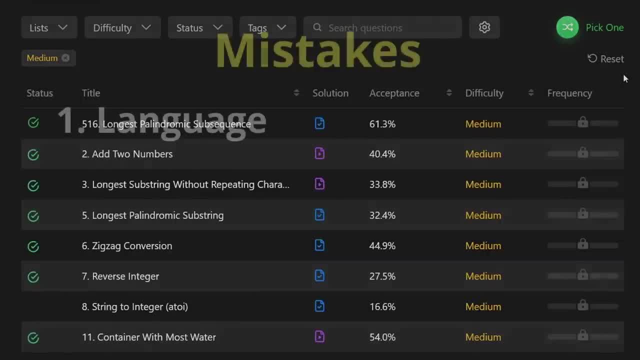 not 50 problems was enough for me to get an internship at a bank. But I knew I had to keep grinding if I wanted to get a job at a big tech company. So I continued to solve problems in a random order, which was another mistake. But probably 60 or 70 questions in I switched to. 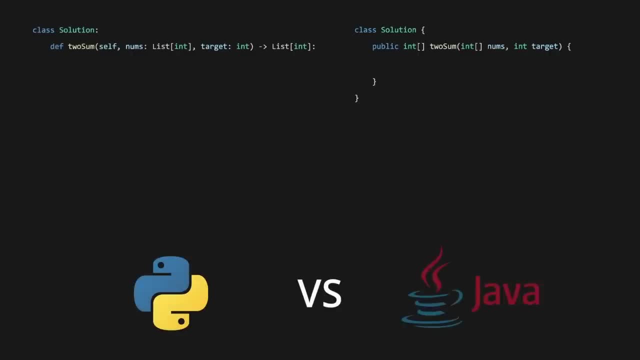 Python. I would have been able to solve a lot of these problems if I had a job at a big tech company. I would always look at the LeetCode Discuss section and I saw that Python code was always the shortest and most concise. Even though I had never used Python before and still to this. 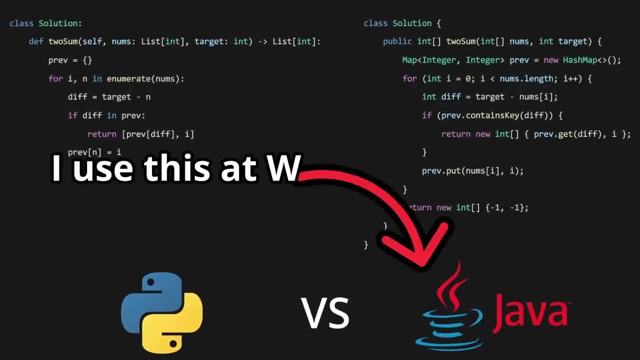 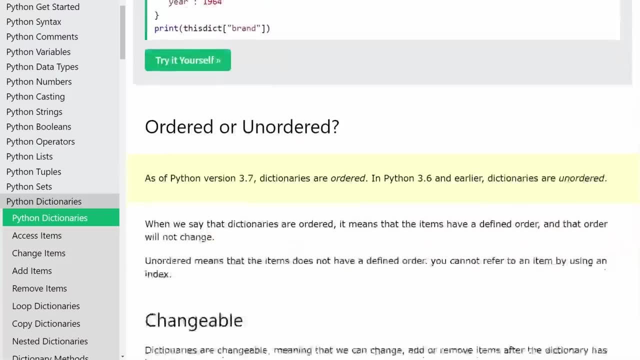 date, I've never used Python at any job or internship. it was an easy choice to make because you don't have to learn the entire language. You really just have to learn the basic syntax: how to write if statements for loops and all the standard data structures. 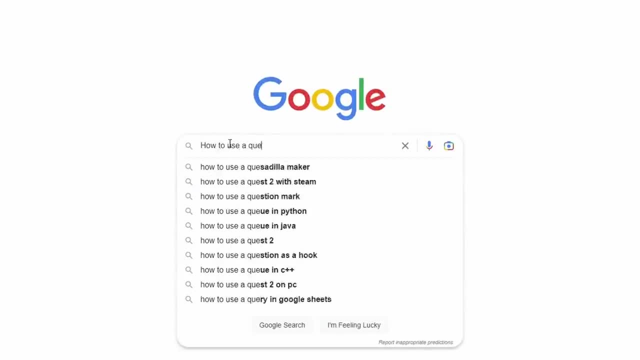 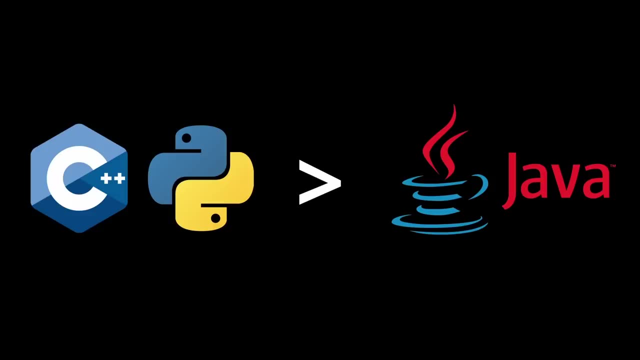 and methods, And you can actually learn these as you solve LeetCode problems just by Googling as needed. Now, C++ isn't a bad choice either, but I would definitely avoid a verbose language like Java. The language probably won't be a deal breaker, but it can. 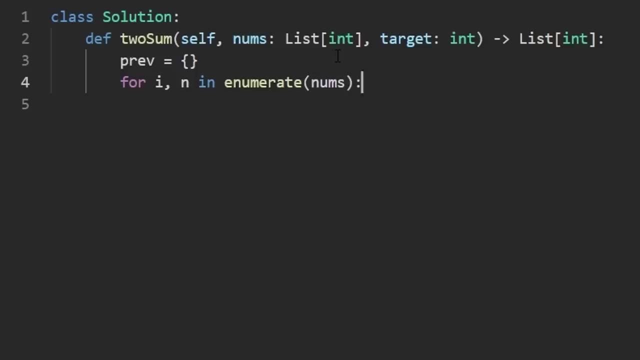 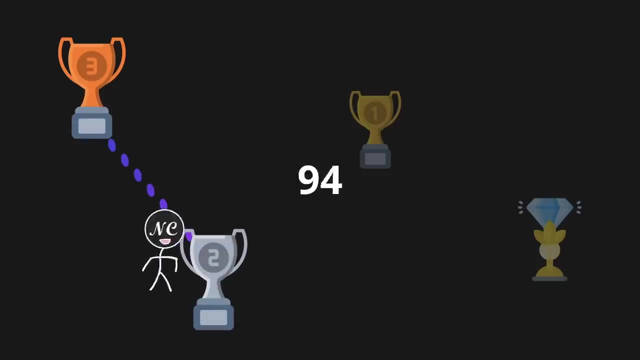 definitely save you a few minutes when you're typing out your code, which can definitely make a difference in a real interview. But it doesn't matter how fast you type if you can't actually solve the problem. And even after solving 100 problems, while I had learned all the high-value. 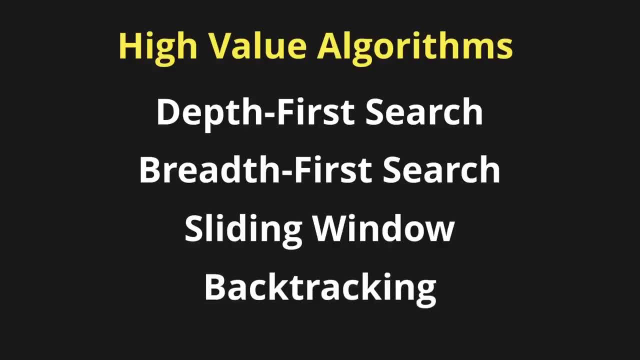 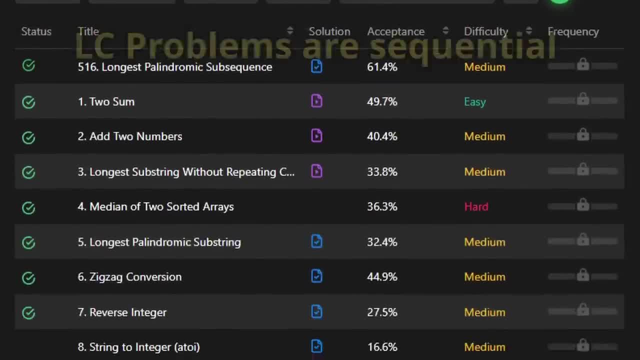 algorithms like DFS, BFS, sliding window and backtracking. I wasn't able to consistently solve a new problem for the first time. I didn't know it then, but the reason was that a lot of LeetCode questions are sequential. You've probably seen questions like House Robber 1,, House Robber 2,. 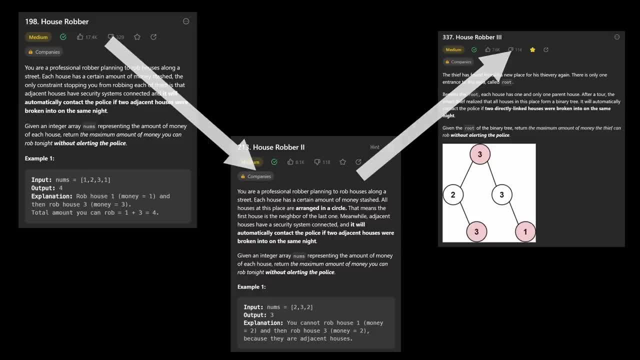 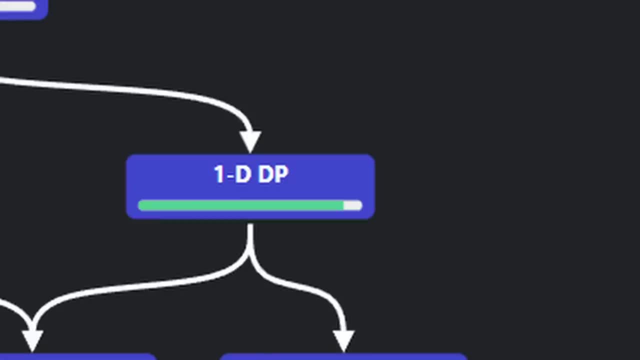 and House Robber 3. Obviously you should solve these questions in order, But actually most of LeetCode questions should be solved in a specific order. For example, you should never try solving dynamic programming problems unless you already have a solid understanding of. 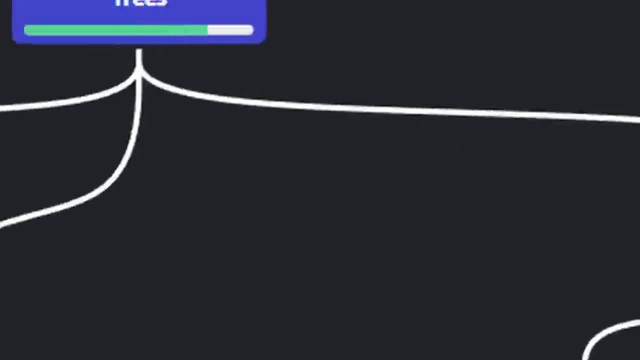 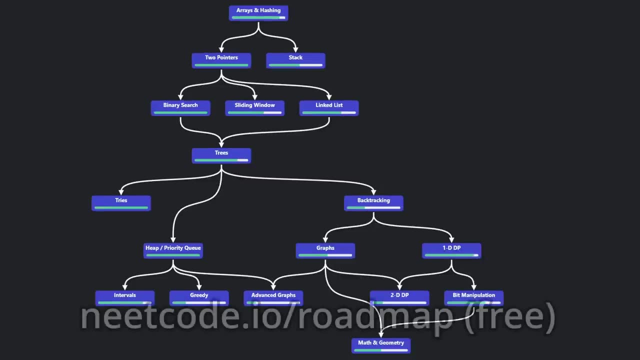 backtracking, And you probably shouldn't try solving graph problems until you have a solid understanding of trees. This is obvious in hindsight, but I'm sure a lot of people make this mistake, which is why I created a roadmap for LeetCode. So let's get started. 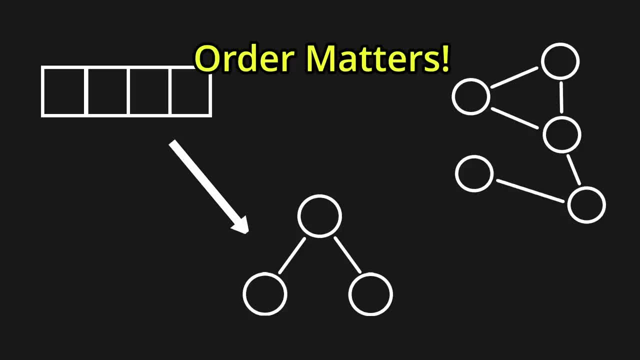 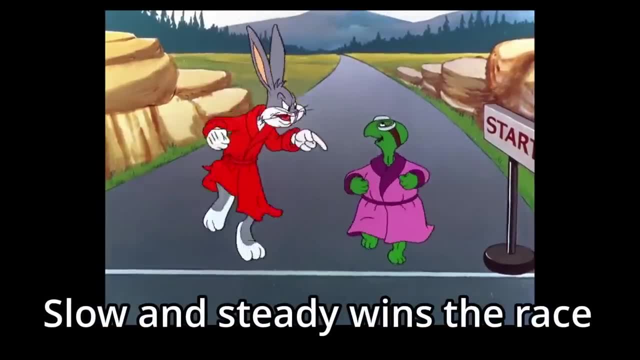 I'm going to start by explaining the order in which you solve problems in the map, so that you don't make the same mistake I did. It turns out that the order you solve problems in does matter. I also think that solving one or two problems a day consistently is a lot better than cramming. 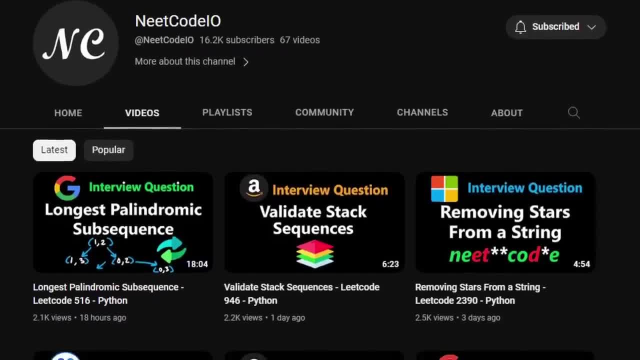 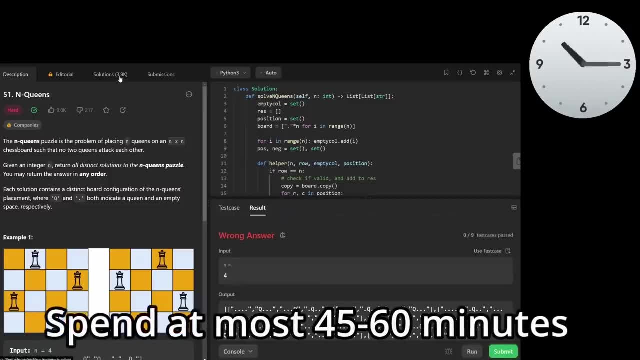 because the ideas will actually stick If you need a little motivation. I've been solving daily LeetCode problems on my second channel. As I continued, I realized that if I couldn't solve a question in 45 to 60 minutes, I wasn't going to be able to solve it myself. Previously I would literally 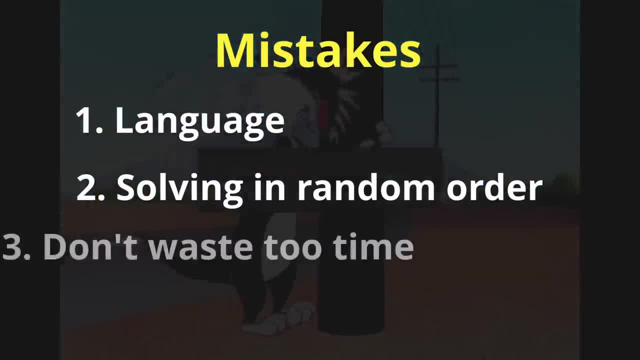 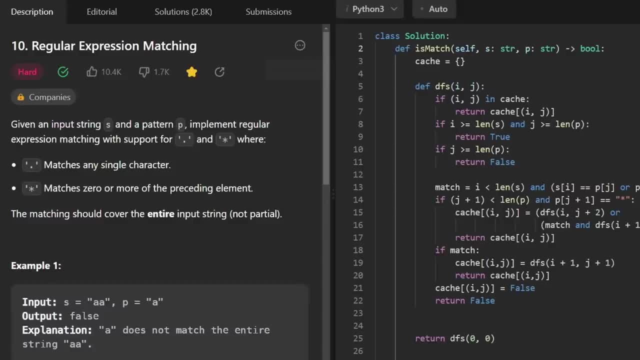 bang my head against the wall for 3 to 4 hours on a single problem because I thought that was the only way to learn. But let's just be honest: most of us are not going to be able to come up with some of these complex academic algorithms by ourselves. And even if you can come up with, 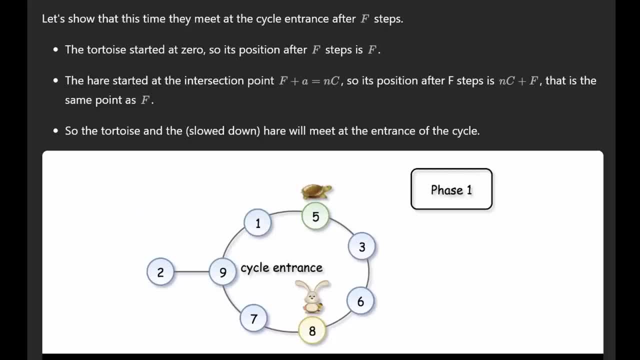 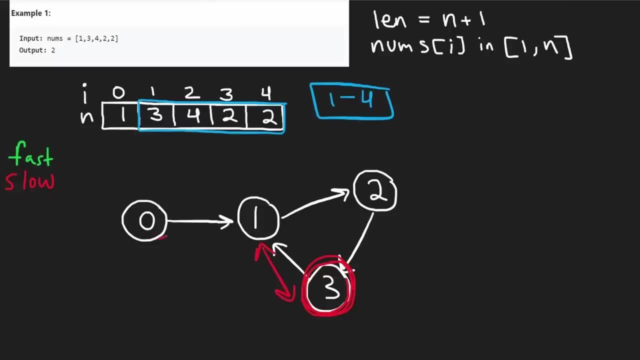 Floyd's tortoise and hare algorithm. it's probably not an efficient use of your time. There's no shame in looking at a solution, as long as you can understand exactly why it works. That's why in my videos I really try to explain my thought process behind every problem. 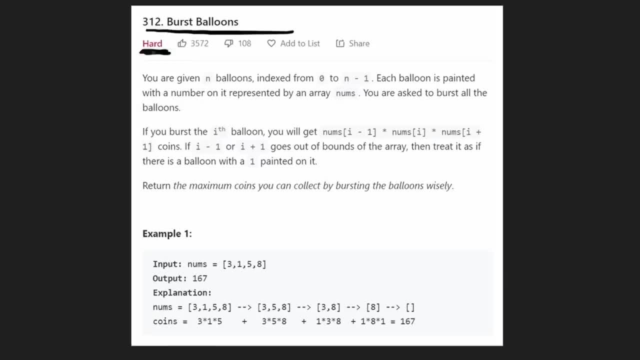 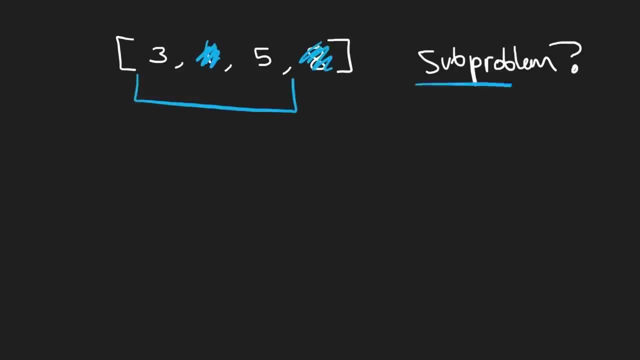 This ended up saving me a lot of time, because I would get to a really hard problem, a crackhead problem- I like to call them like burst balloons- and I would get pretty close to solving the problem. I would know it's a dynamic programming problem, but I just couldn't figure. 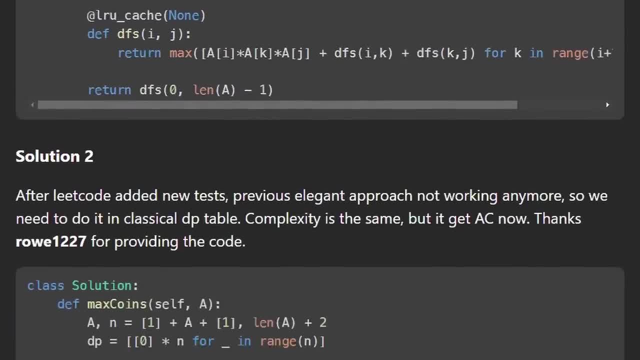 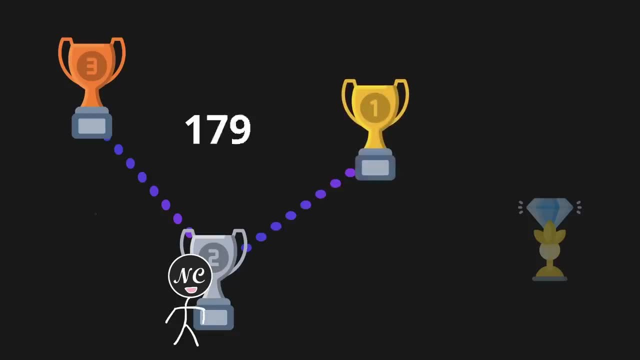 out the trick behind it. Then I would look at a solution and only after 5 minutes of reading I would realize: oh, that's the trick, and then I would be able to immediately solve the problem. I was able to go from 100 to 250 solved questions a lot faster than I was able to. 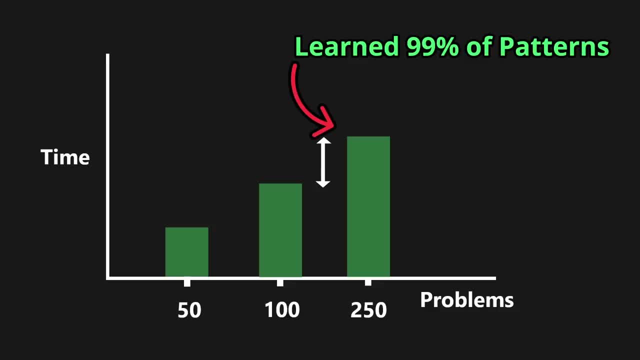 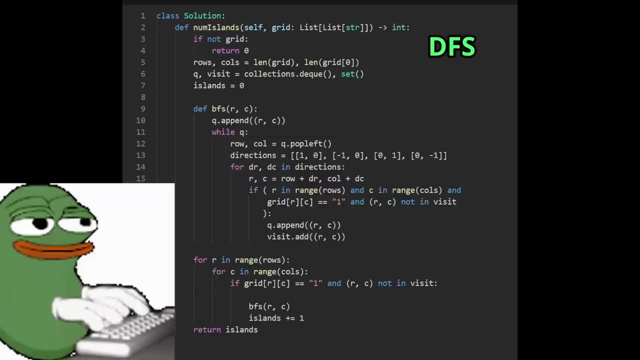 solve my first 100 questions And by then I had learned 99% of the patterns that I needed, even some of the complex ones, And I got to the point that writing out these algorithms like DFS, BFS and binary search was as easy for me as writing a for loop, Even some advanced ones. 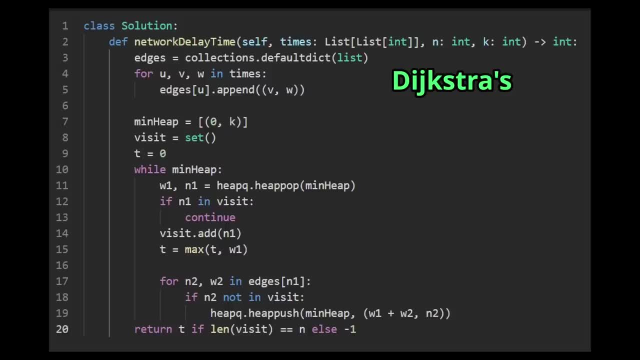 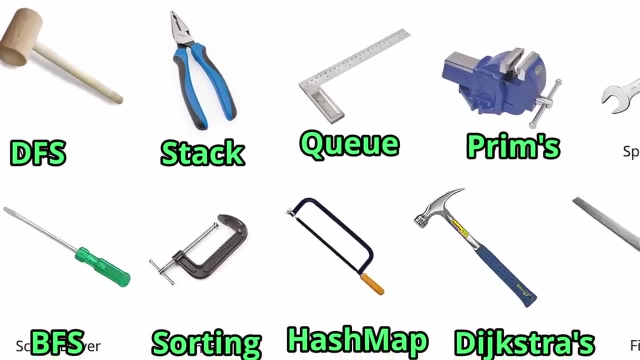 like union find Dxtras I could write out in less than 5 minutes, And that's when I realized that most leak code problems fall into these buckets. For medium questions, you just need to figure out what algorithm you need and then apply it. Hard questions are similar. 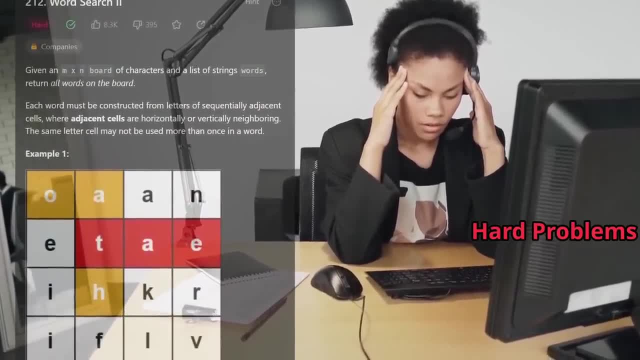 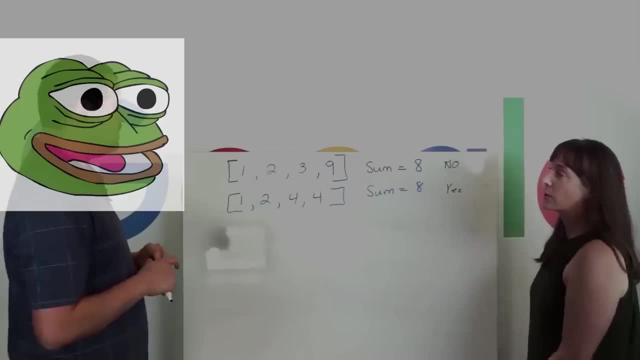 except there's usually a really complex trick behind them And sometimes, unless you've seen it before, only God can help you figure it out, Or maybe your interviewer, if they happen to be generous. At this point I was confident I could pass interviews, but I wasn't 100% sure if I was. 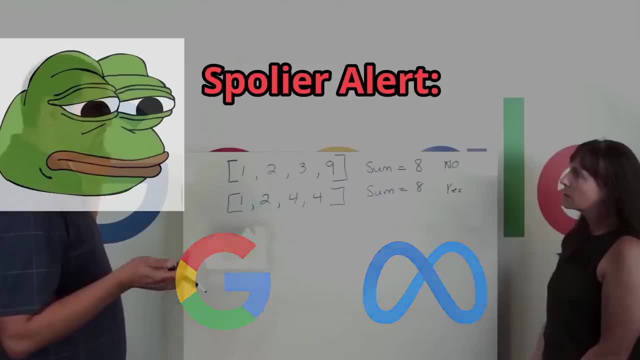 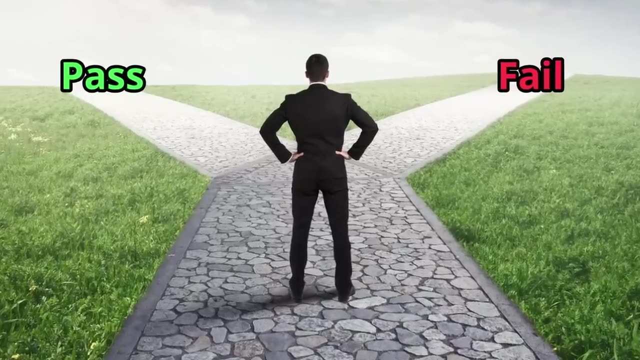 ready for the big tech interviews like Google or Facebook. And spoiler alert, you will probably never feel 100% prepared. It's not a binary decision whether you are ready for an interview or not, because you never know which questions you're going to be asked. It's more of a 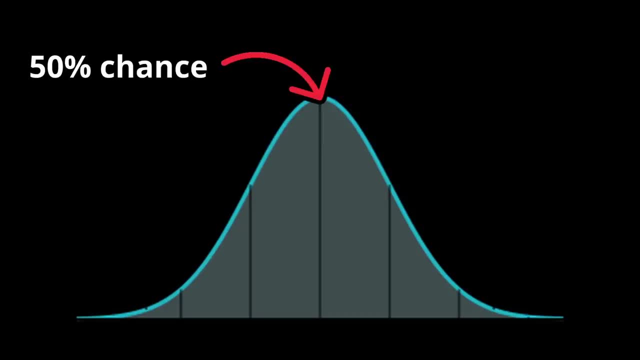 distribution. You might have a 50% chance of passing, or you might get to the point where you don't. If you're a perfectionist, I'm sure you want a 100% chance, but that's almost never going to be the case. I think a good rule of thumb is that you should be able to solve a medium problem. 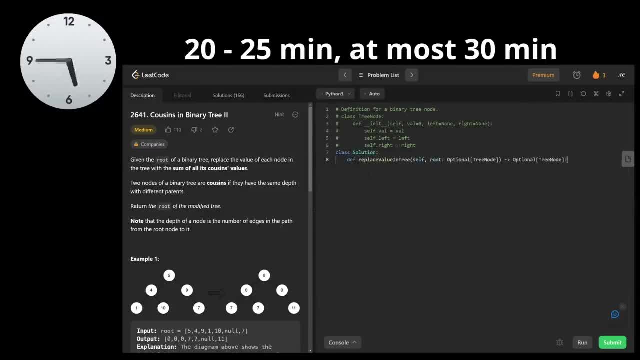 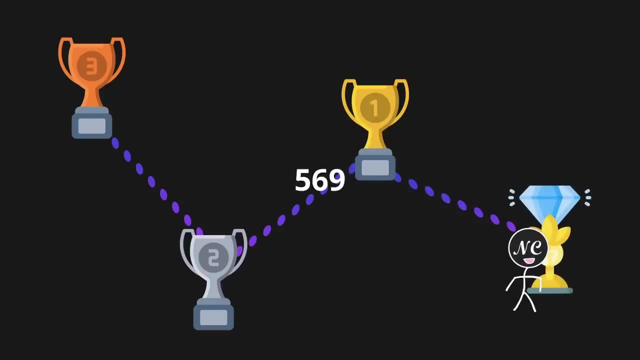 that you've never seen before in 20 to 25 minutes. If you can do that, you probably have at least an 80% chance of passing most FAANG interviews. And I continue to solve up to 569 problems even though I had already gotten into Google, mostly because I'm a loser, But it's not quite. 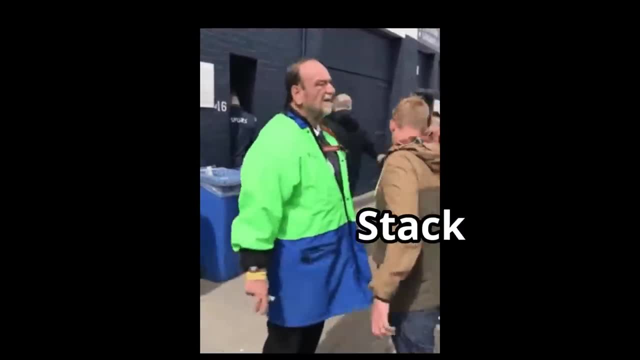 as time consuming as you might think, because I've gotten to the point that I can solve most medium questions in 10 minutes. But I'm not going to be able to solve most FAANG questions in 10 to 15 minutes. But I definitely don't recommend it because there are diminishing returns on 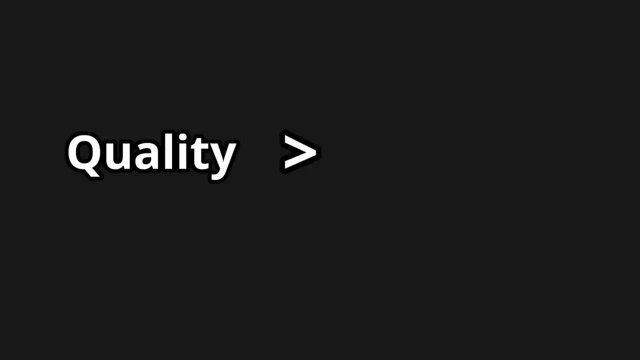 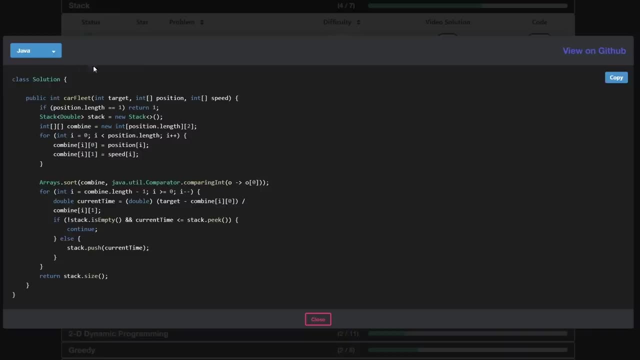 solving more and more problems. I think quality is much better than quantity. I recommend solving about 150 questions, like the Neat Code 150 list, which has video solutions and code solutions in 14 languages, But make sure you really understand each and every problem. A huge mistake that. 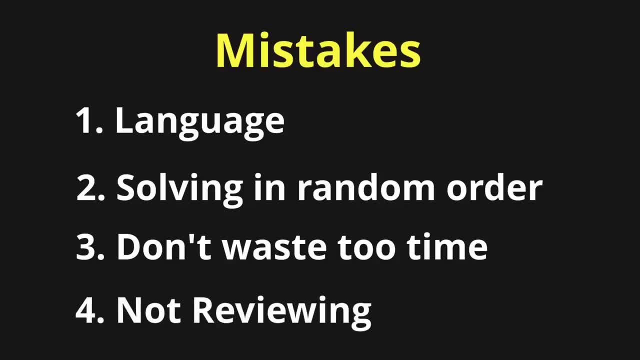 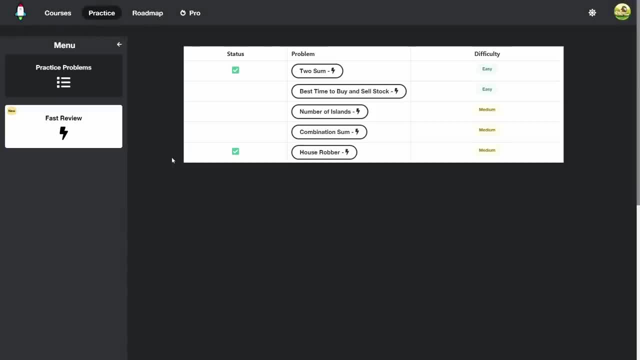 most people make is that they don't go back and review previous problems. For these complex algorithms to really sink in, you need repetition. That's why I'm working on taking each problem from the Neat Code 150 list and converting it into a multiple 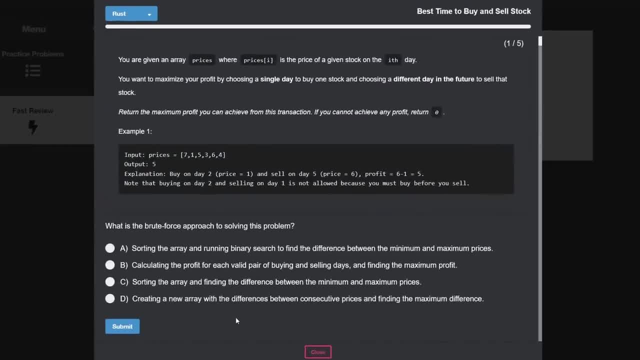 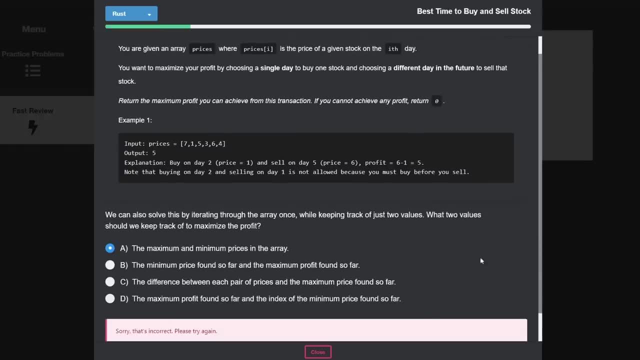 choice quiz, Because it's really hard to go back and re-solve each question and usually all you need to do is review the trick. So I made quizzes that you should be able to solve in a few minutes but also get a lot of value from it. You can check out a handful of problems right now.